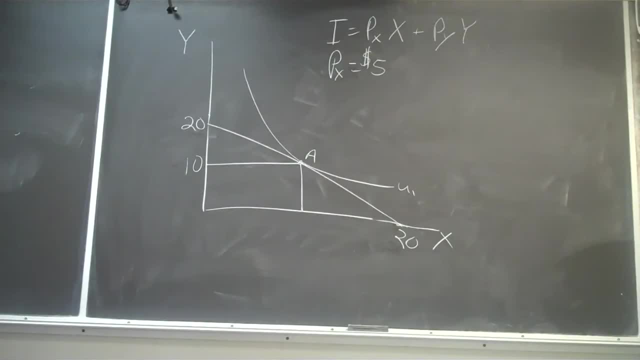 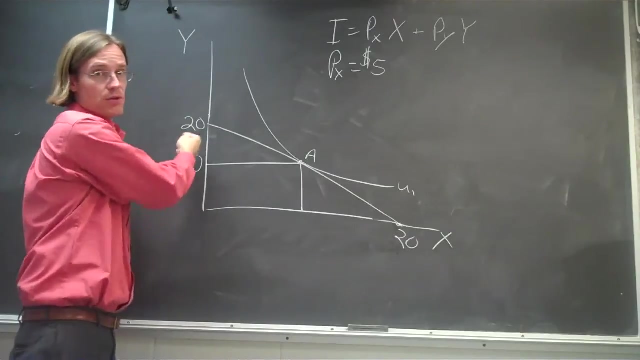 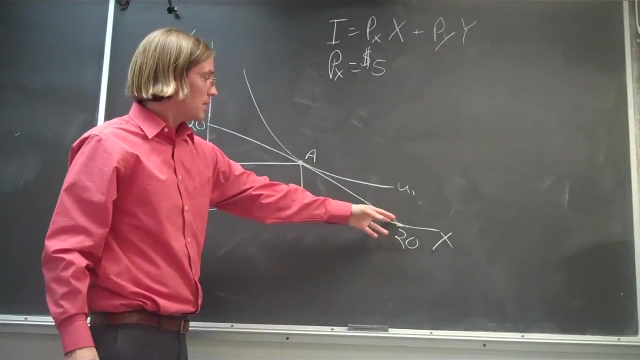 Do a problem here with the budget set of a consumer. So consumers limited to buying two goods: good Y, good X. They can buy 20 units of good Y if they spend all their money on good Y. They can buy 20 units of good X if they spend all their money on good X, Or they can buy some linear combination of the two. 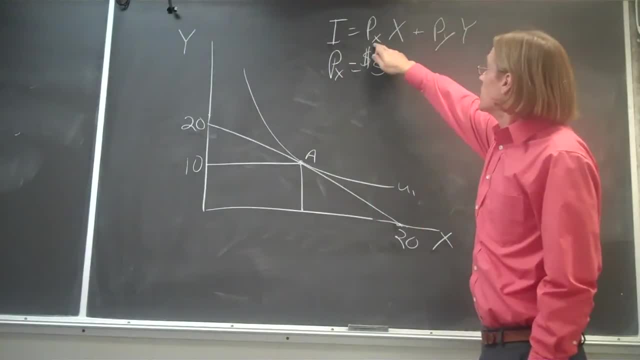 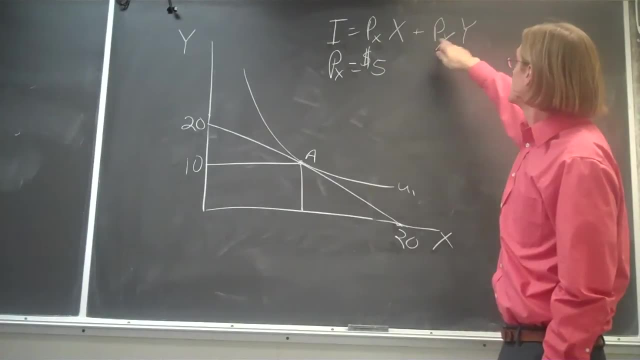 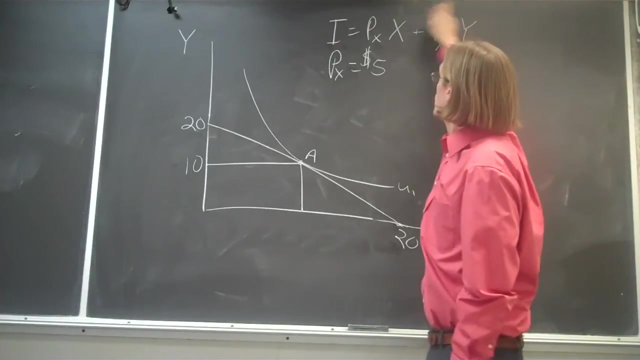 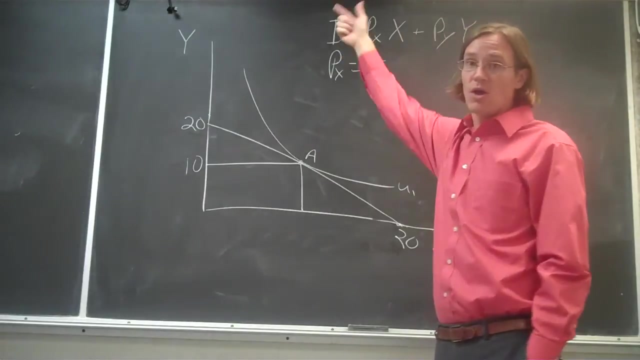 Our income is determined by the amount of good Y. the amount of good X we're going to buy and the price of good X, plus the number of units of good Y we're going to buy, times the price of good Y, And so this is the amount of money we're spending on good X and the amount of money we're spending on good Y. summed together will be all of our income. If we spend all of our money, then we're on this budget line. 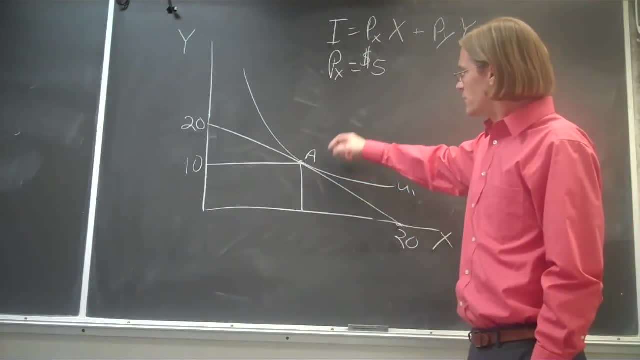 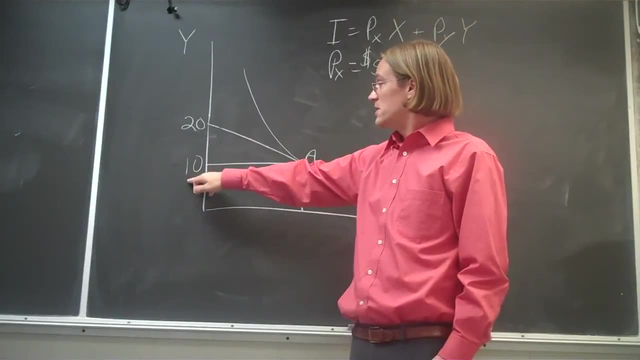 And we can look at this first example here. We're at point A, Then we're spending 10 units. Well, we're spending our money to purchase 10 units of good Y, but we don't know how many units of good X we're purchasing. 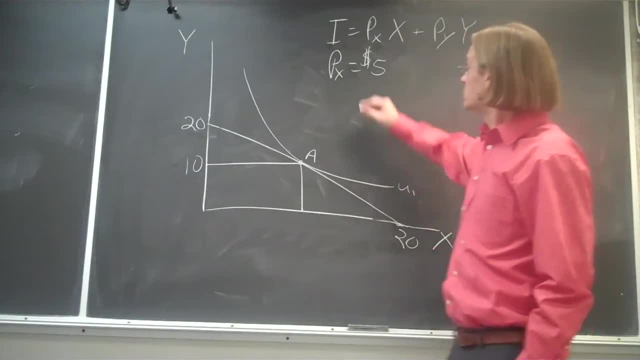 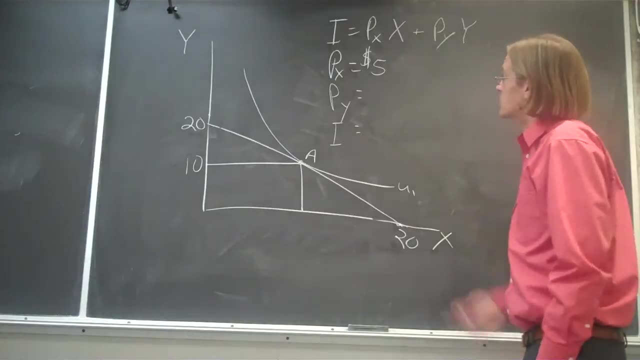 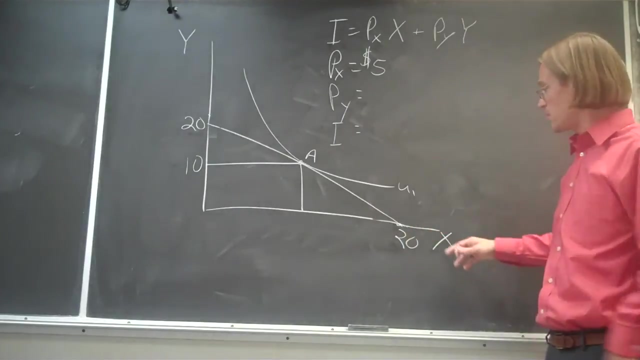 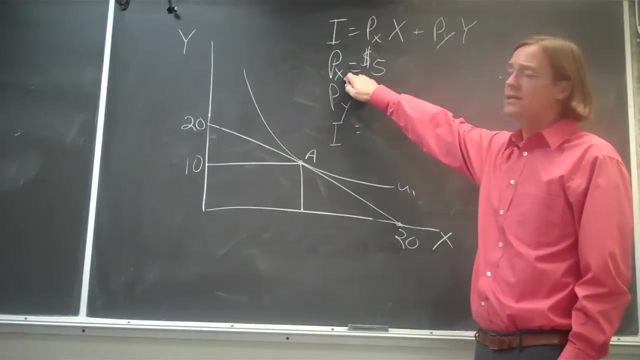 So to do that, we need to go in and figure out a couple things. We need to figure out what the price of Y is and what our income is, And to do that, we can first assume that we're purchasing. So we're purchasing all good X, So we're spending all of our money on good X. We're going to be at this point purchasing no Y And we know that the price of X we're given the price of X is 5 bucks. 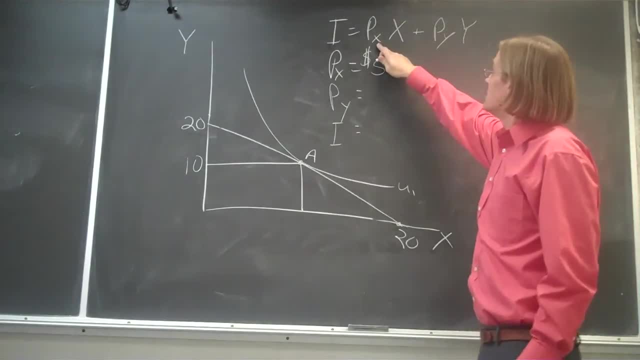 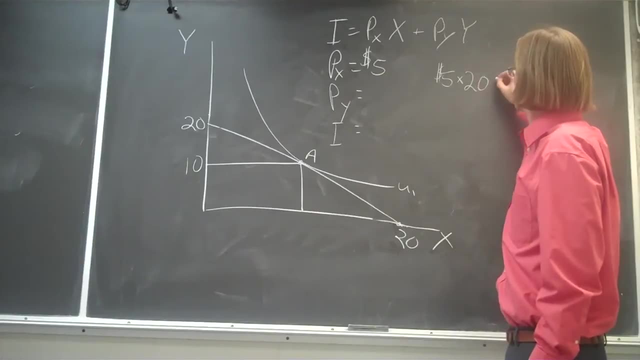 And if that's the case, the price of X is going to be 5 times the 20 units that we're purchasing, plus the price of good Y, which we don't know. But we do know that at this point we're buying no Y. 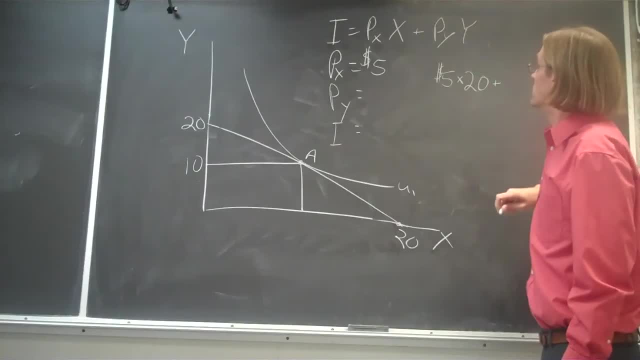 And so we know that this part of the budget constraint is going to be 0. And so that's equal to our income. So 5 bucks times the 20 units is going to be equal to our income, which is equal to 100 bucks. 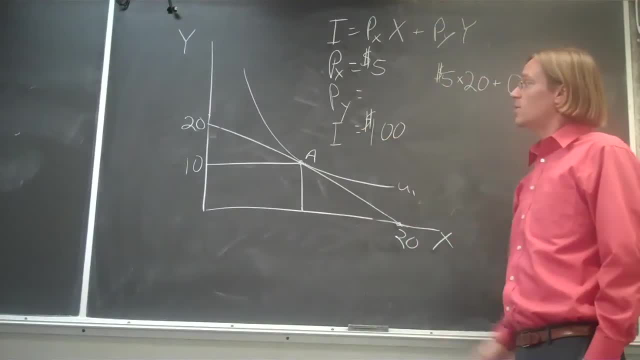 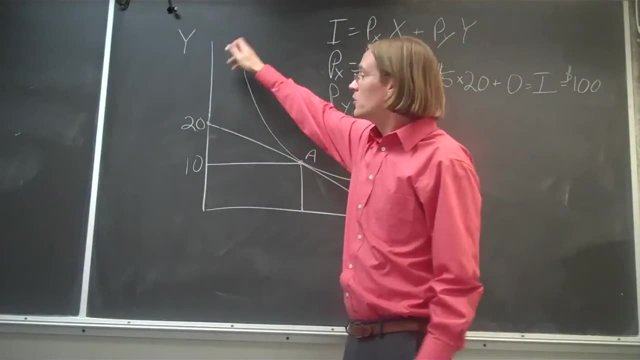 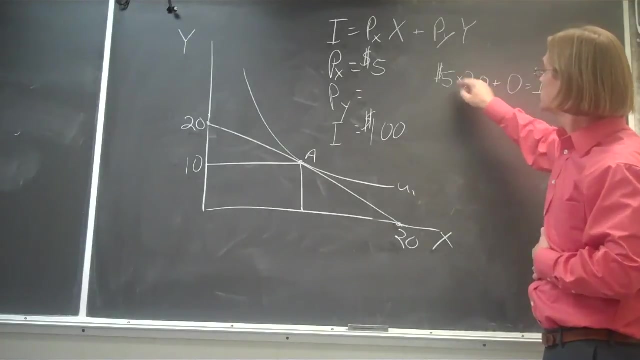 So now we can go back and figure out the price of Y if we go to the other end of this budget constraint and say: you know what, let's assume now we're spending all of our money on good Y. Well, if that's the case, then we're not going to be buying any of good X. So this is going to go away. 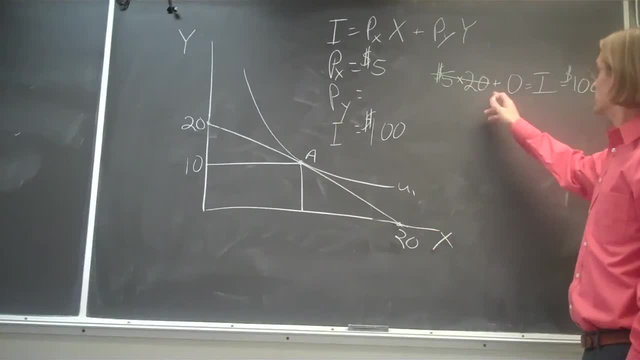 We know that the number of X goes to 0. Don't have to worry about that, But now we have to deal with Y, And so we don't know what the price of Y is. but we know that the price of Y times the number of units of Y that we're purchasing. 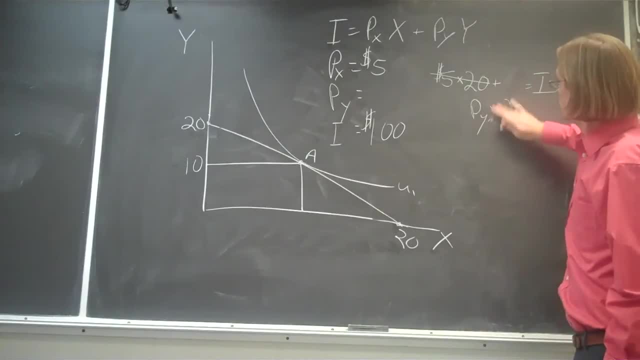 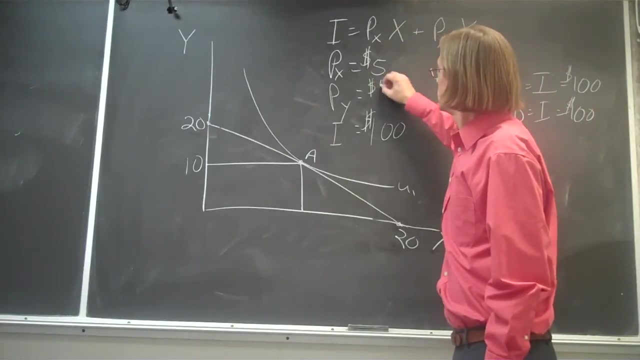 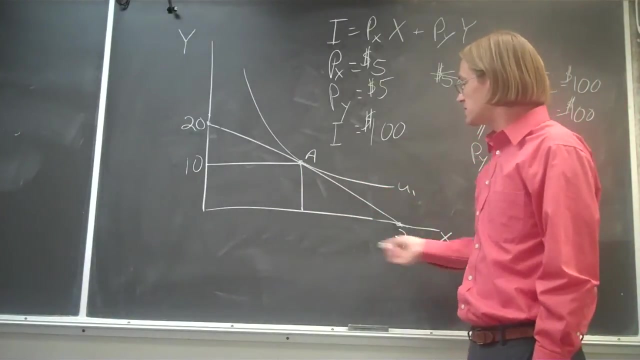 that should be PY. So Y times 20 is going to equal our income, which is equal to 100 bucks, And so from that we can do some really high-end algebra to show that the price of Y is 5 dollars. So now, if we're at point A, how many units of X can we purchase? 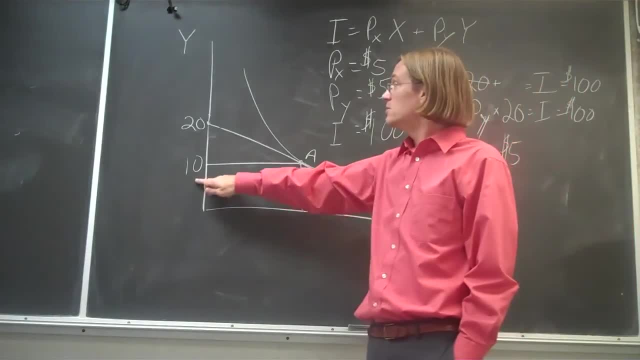 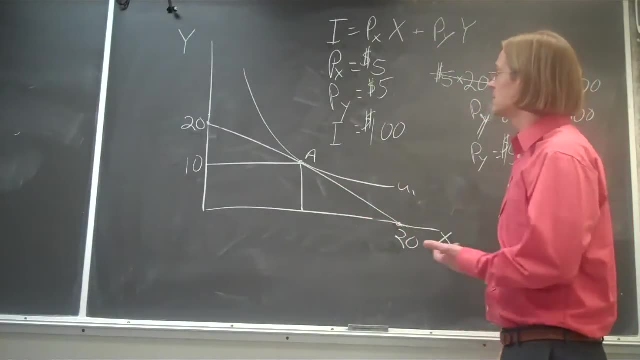 Well, if we've got 100 bucks And we're buying 10 units of Y at 5 dollars apiece, then we've got 50 bucks left over, And if the price of X is also 5 dollars, then we use that 50 bucks to buy good X. 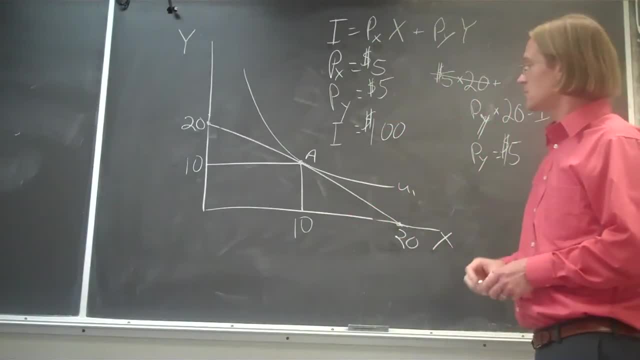 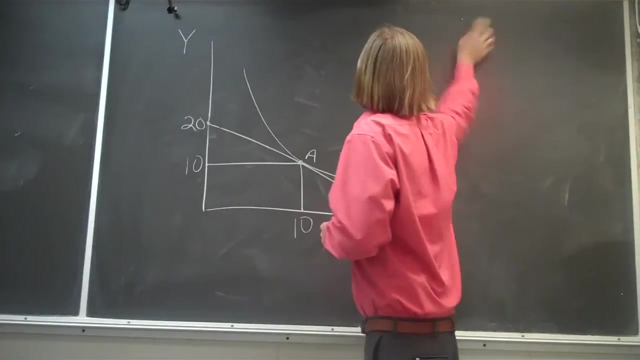 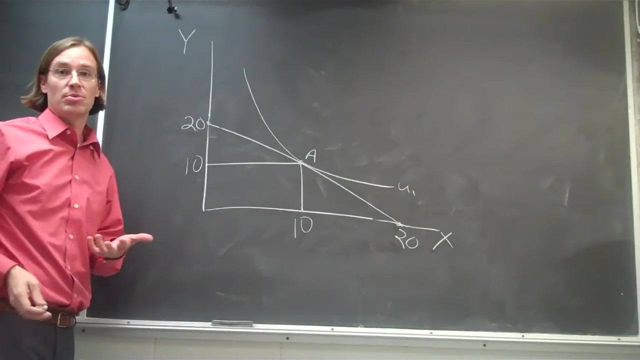 And we should be able to buy 10 units of good X. What happens now if the price of Y changes? So Y has been 5 dollars. Now you go into the store and all of a sudden you're fired up because one of the two goods that you purchased just decreased in price. 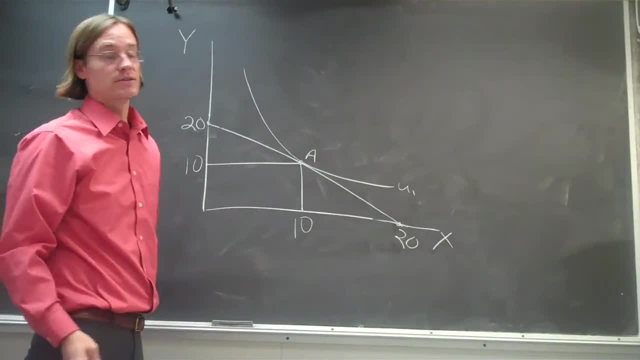 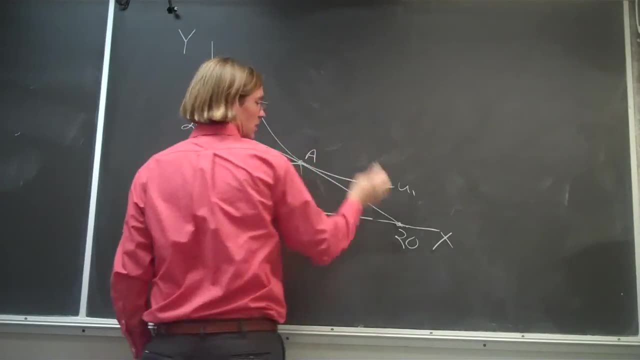 So if Y went from 5 dollars to 2 dollars and 50 cents, we're going to see this budget constraint, this budget set, rotate around this point. Nothing's changing about X. Nothing's changing about X. The price of X isn't changing. 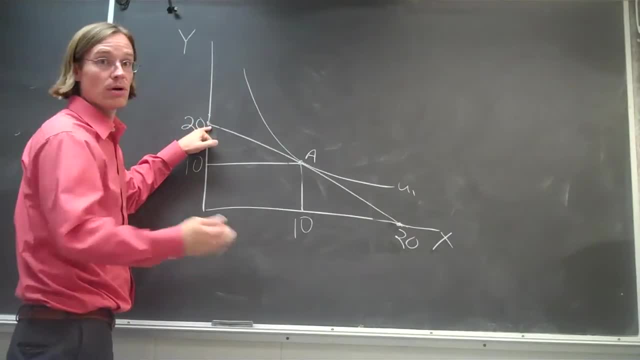 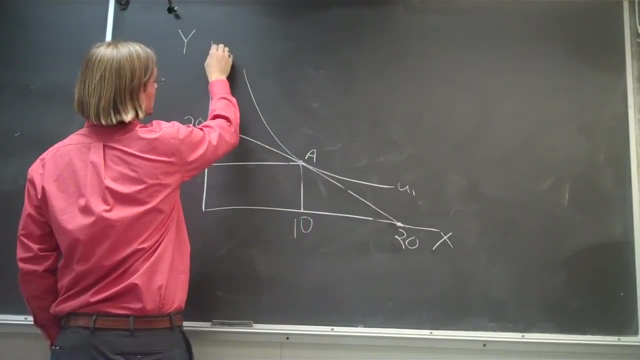 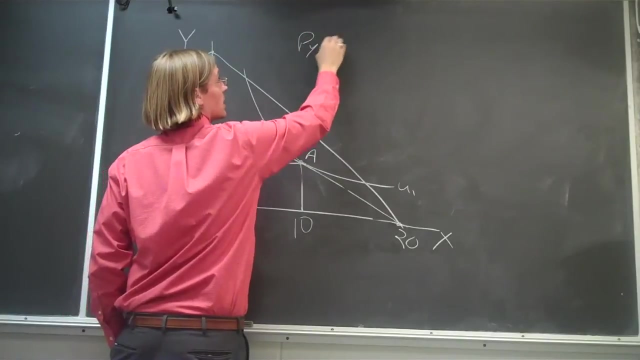 But as the price of Y drops, you know you can buy more of good Y And so this budget line rotates. So let's say it goes. if the price were cut in half, the price were cut to 250.. So our new price for Y: 2 dollars and 50 cents.